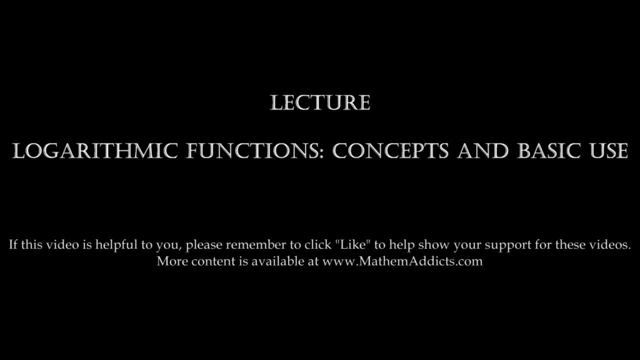 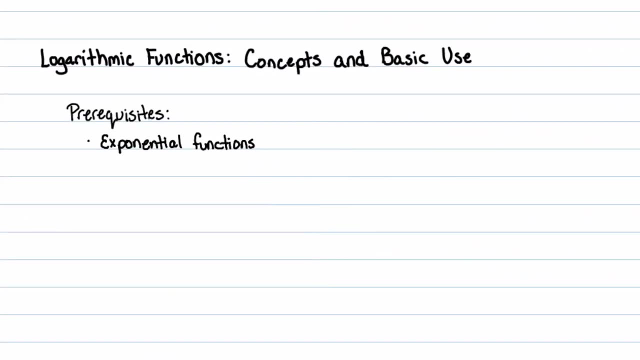 We now approach a topic that a lot of students kind of shy away from when they first are introduced to it. but in reality this topic is not so bad if presented correctly. I don't know if I'm going to be the one who presents this correctly, but I'll try. This is all. 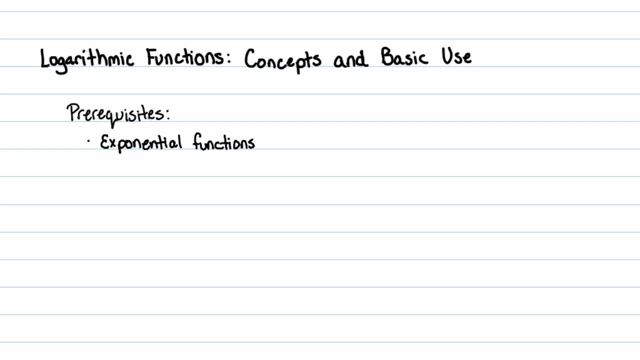 about logarithmic functions, their concepts and basic use, And the only prerequisite here really is an expanded knowledge of exponential functions. You should be pretty familiar, actually very familiar, with exponential functions. We are uniquely- actually not uniquely- we are faced with a new problem, And what I mean by a new problem is that every time you learn, 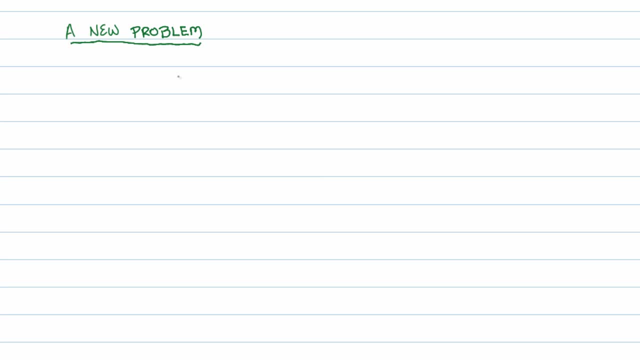 something in the past like how to solve an equation. you're faced with a new problem. You usually- no, always- use inverse operations to solve that equation. In other words, if somebody came along and said I need you to solve this, x plus 3 is equal to 7, you would 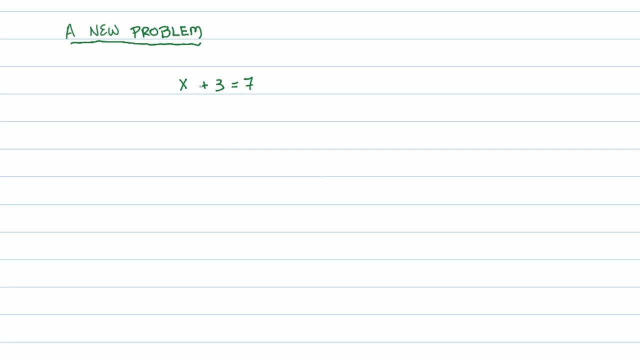 say: ah, I need to subtract 3 from both sides. That's because you're doing the inverse of what 3 is doing to the left-hand side. So the inverse of addition would be subtraction. So you'd subtract 3 from both sides, And when you do that, this equation becomes equivalent. 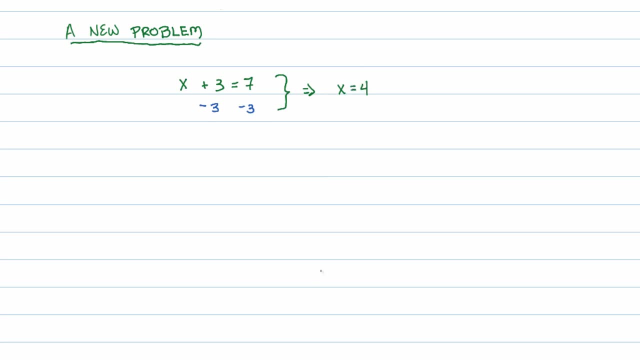 to x equals 4.. And all of a sudden you have the solution. Well, what about if somebody came along and handed you: 3x is equal to 7?? Again, you're thinking: OK, I know how to do this, I just divide both sides by 3.. Well, really, how you should think about it is 3. 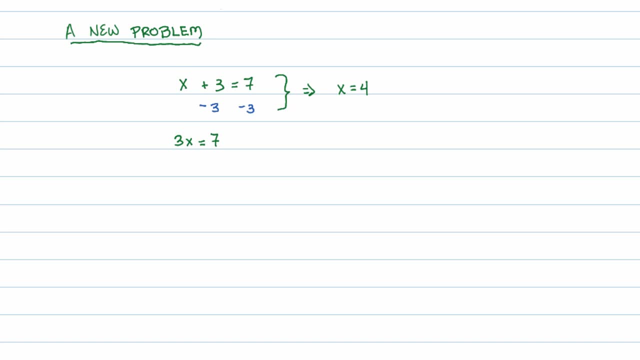 is multiplying x. How do I undo that? How do I do that? Well, you're going to have to do multiplication. You undo it with division, So you divide both sides by 3.. And notice, if you've watched all my lectures, I've been very much focused on teaching this idea throughout. 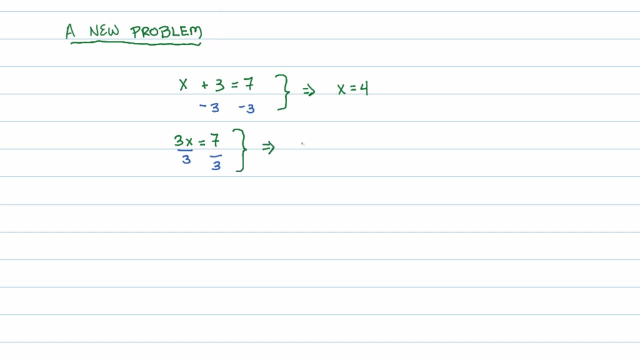 this lecture series of doing the inverse of what's happening to x: undoing or untying the knot. So in both these cases we knew what to do. Same thing. if I give you 3 times, the square root of x is equal to 7.. 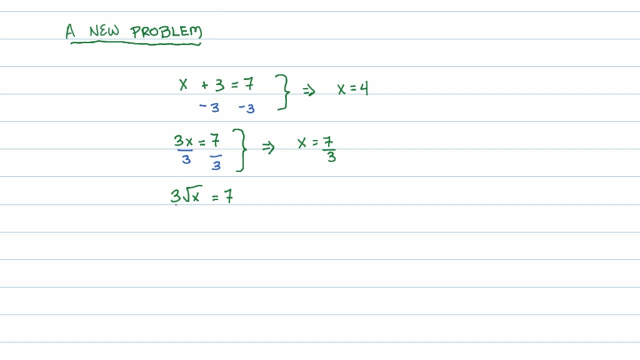 Well, a lot of people say: OK, first I'm going to divide by 3. So I could go ahead and do that. Let me just put that middle step in here, And then I'll get an equivalent expression or an equation, I'm sorry. which is the square root of x is equal to 7 thirds. And now how? 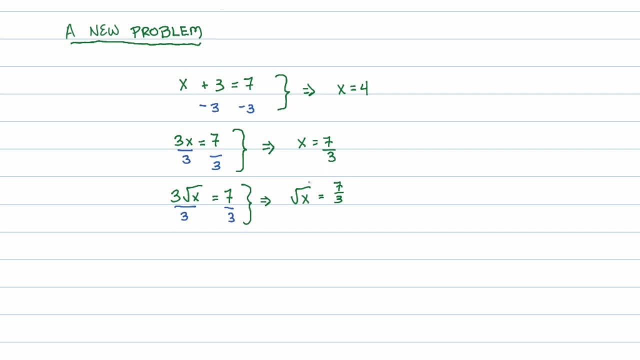 do you undo a square root? You square both sides. So each time I'm just looking for x. So this implies that x is equal to 49 over 9.. Not much else I could do with that, And more recently we've dealt with things like x to the 2 thirds is equal to. let's. 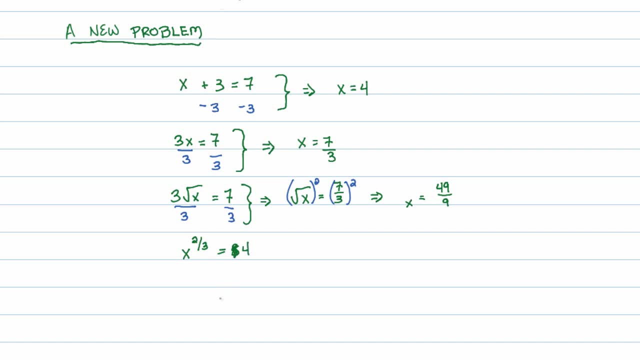 say 8. Or, better yet, let's do 4.. x to the 2 thirds is equal to 4.. Again, you have to think of how do you undo a power of 2 thirds? Well, recently we've discovered that you. 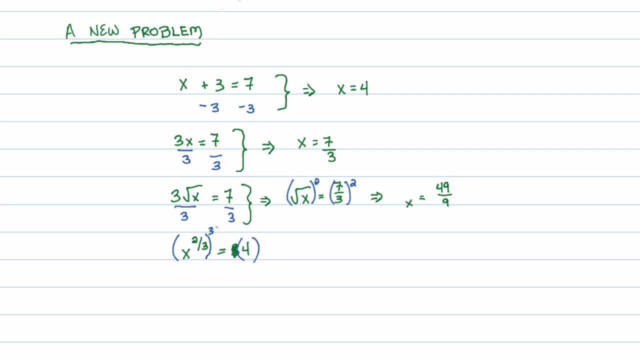 raise both sides Subtitles by the Amaraorg community to the reciprocal power 3 halves. That is the inverse operation. So let's see what happens here. On the left-hand side, powers to powers multiply, So the 2s will cancel, the 3s will. 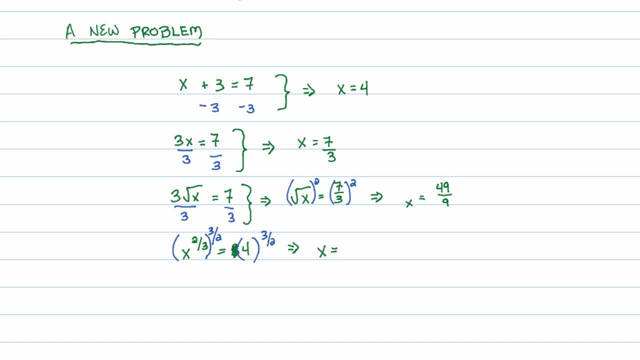 cancel, You'll just get x On the right-hand side. that's like saying the square root of 4, which is 2, to the third power, Or in other words, x is equal to 8.. So you've learned. 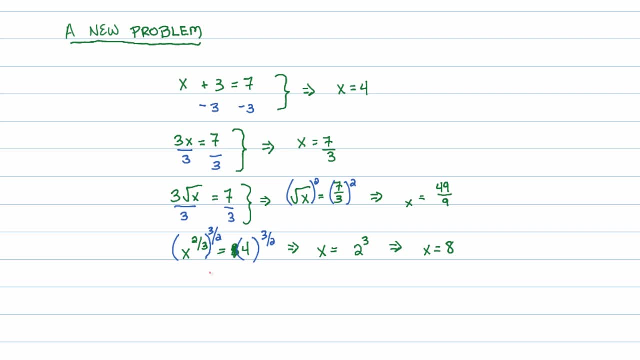 throughout mathematics How to undo operations. In arithmetic you were told you were given addition, and then soon after you were given subtraction, And then also in arithmetic you were given multiplication soon after you were given division, And then in pre-algebra you were given powers like 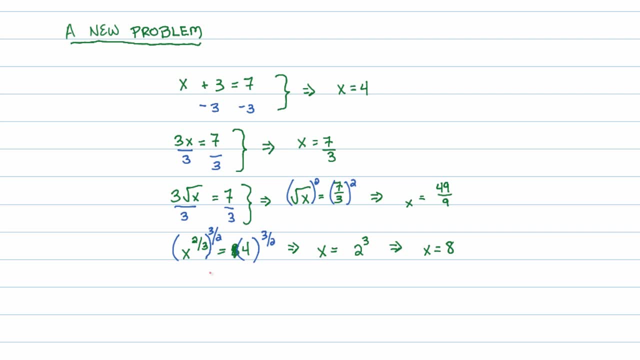 the squaring something and eventually you got to square roots, which would undo squaring something. In algebra, you have raising something to a fractional power or rational power and you undo something. So you have to do something. And then in algebra, you have raising something. 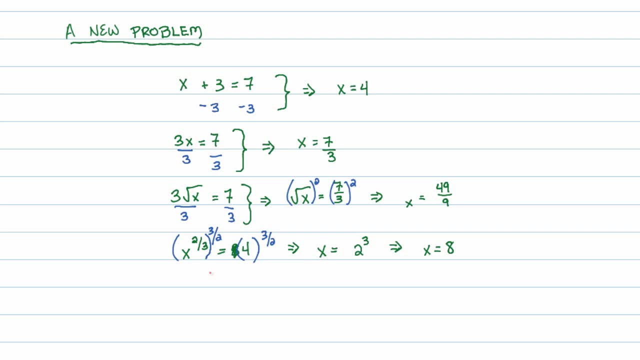 to a fractional power. So you have the right-hand side and then you're given the right-hand side and you're given the right-hand side and you have the right-hand side. So you have to do it with the reciprocal rational power. But what happens when we now have a new concept? 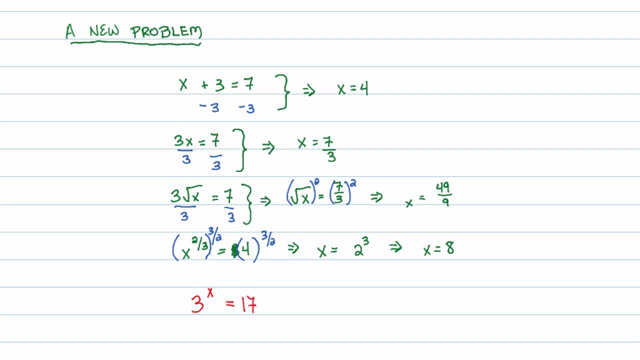 called an exponential equation and you want to solve something like this. What undoes a variable being raised to some base Or raised by some base? Basically, how do you get a variable out of an exponent? I've never had a great way of saying that, by the way, But 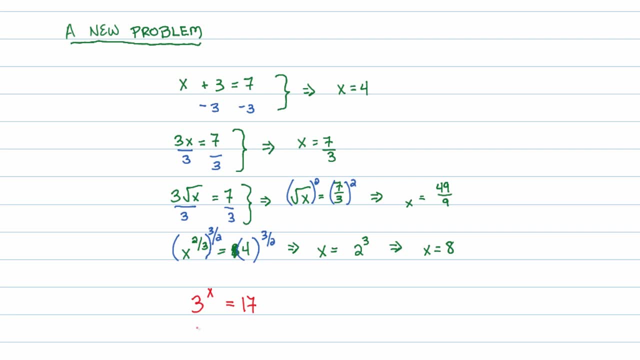 how do we undo something? How do you get a variable out of an exponent? You have to do it with the reciprocal rational raising x into the exponent. well, now we have to create something new again. always think about the fact that subtraction was really created to undo addition, and division was really created. 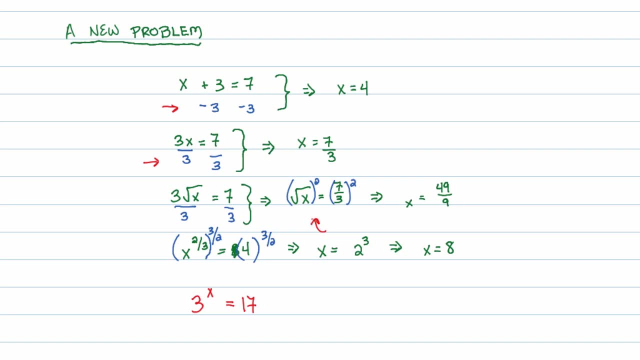 to undo multiplication and squaring- you can think of as being created- to undo square roots and so on and so forth. so we need to create a new object to undo this, to get x by itself. so enter the logarithm, the base b, logarithm of x, written as log sub b, that little b is. 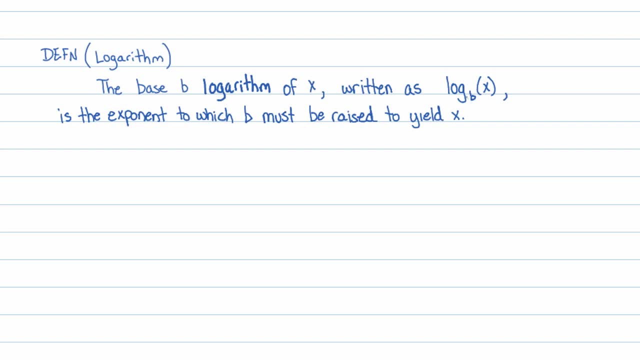 just written slightly below the the line i guess you could say of x. so log base b of x is how most people say. that log base b of x is the exponent to which b must be raised to yield the logarithm of x. and i've never really liked this definition because it's very difficult to digest, it's much. 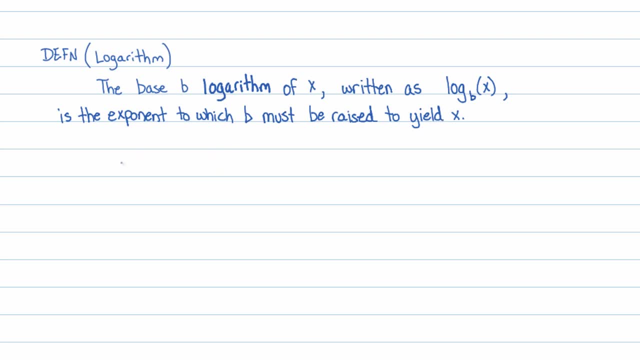 easier to see it when somebody actually writes out its equation equivalent. so let me do that. all right, that is, y is equal to log base b of x, if, and only if, b to the y power is equal to x, b to the y power is equal to x. 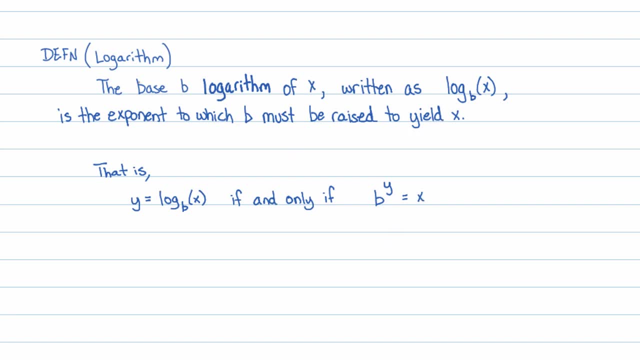 x. so if you read this sentence up here and compare it to this statement, this exchange statement down here, we'll see if it works out. the base b- logarithm of x of the base b- logarithm of x, that's this junk. right here is the exponent. oh okay, so is an exponent. 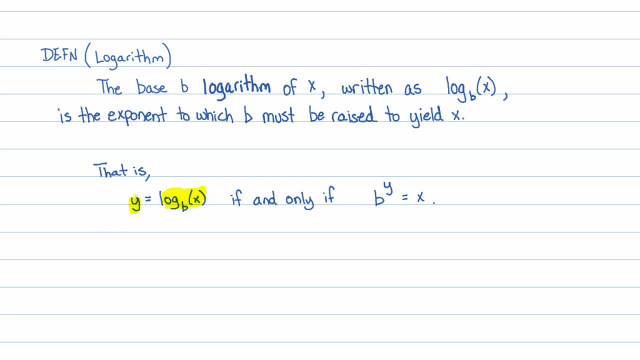 so that's saying that log base b of x is just equal to some exponent value to which b must be raised to yield x. So that's saying that if b was raised to this value, y, it would give us x. And look over here: b raised to the value of y is equal. 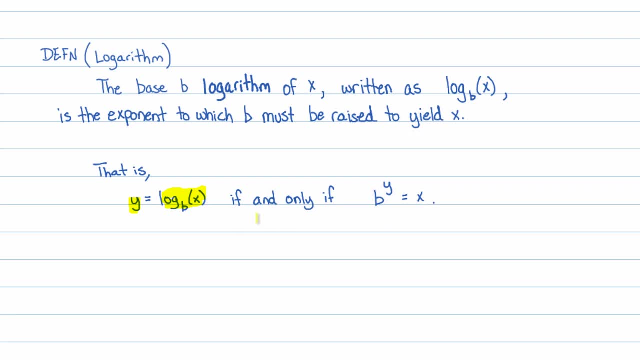 to x. So these two statements are saying the same thing, And I often say it's the circular argument. In fact, I usually don't write y equals log base b of x. I usually write it the other way. I write: log base b of x is equal to y. No real reason other than that's. 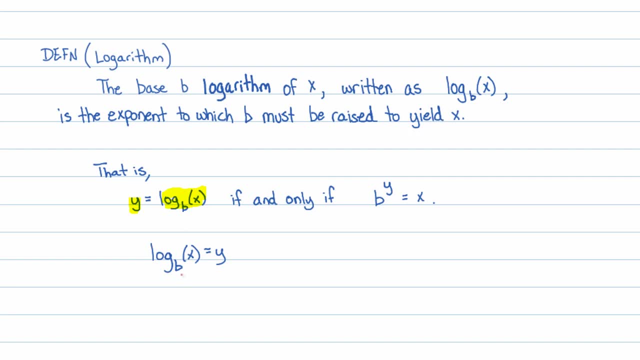 just what I have a habit of, But I use what I call the circular argument. Say that b raised to y is equal to x, And let me write raised to and equal. So b raised to this statement log base b of x is equal to y is the same thing as saying b raised to y is equal to. 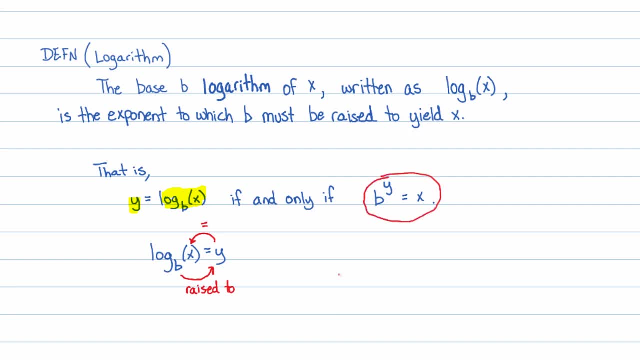 x, And if you look right here, that's exactly what it says: b raised to y is equal to x. Now some people just look at this and get completely flabbergasted. They just don't know what to say or what to do. They're completely lost, Until I remind them that you've actually 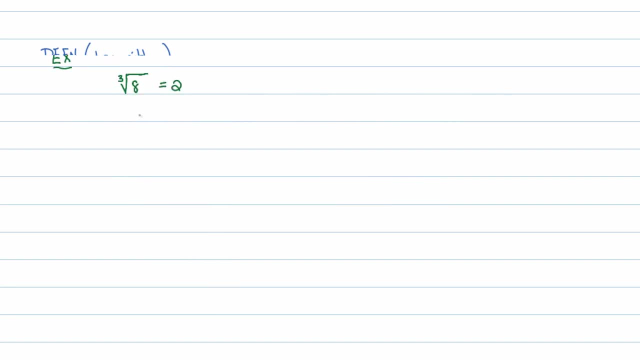 done stuff like this for quite some time. For example, the cubed root of 8 is equal to 2 really means that 2 raised to the third power is equal to 8.. 2 raised to the third power is equal to 8.. So you have seen this. 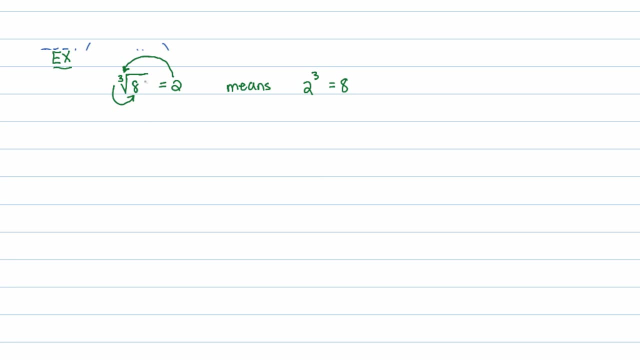 notation before. It's just switching forms. You're switching in this case from a radical equation to an exponential equation. Also, you've seen it in stuff like this: 13 minus 3 is equal to 10 means the same thing as saying 13 is equal to 10.. So you've seen this notation. 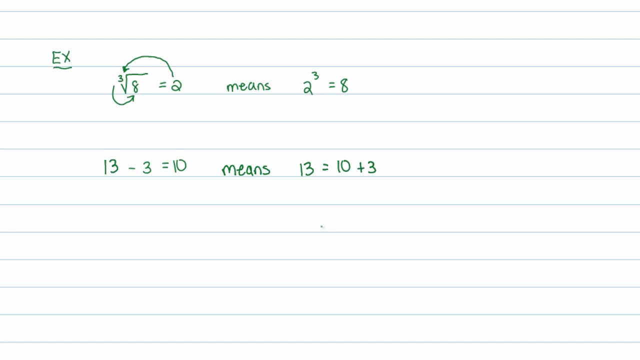 before: 13 is equal to 10 plus 3.. So all I did was say that 13 is equal to 10 plus 3.. It's like this circular argument kind of goes around with everything we know, But the idea is, you've seen this transformation of form quite often, So this idea back here of transforming, 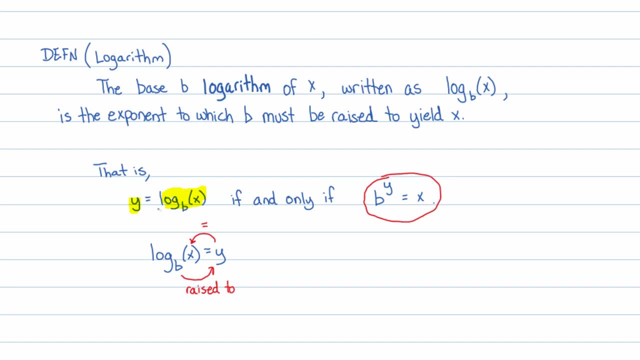 from an exponential equation to a logarithmic equation. you've seen this transformation of form quite often, So this idea back here of transforming from an exponential equation to a logarithmic equation- While it's new, the letters are new the idea of transferring 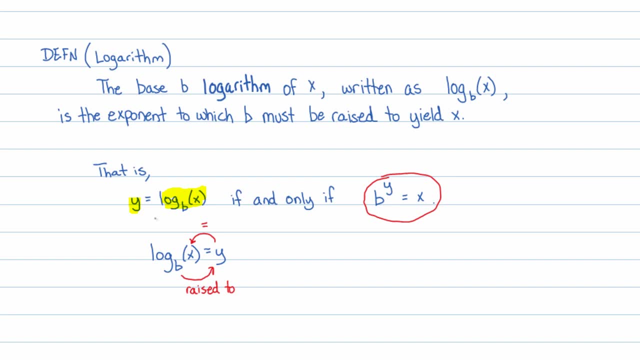 between forms shouldn't be so new. Try to convince yourself of that by kind of rewinding this and taking a look at this example here again, especially the first one. The first one is a great example of switching forms. So let's take a few examples here. Let's rewrite: 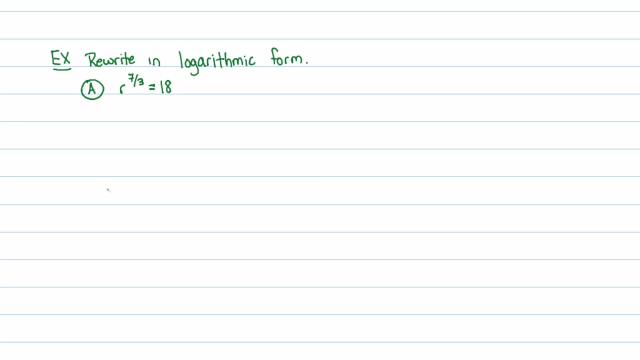 some exponential equations, or in this case, this is a power. Well, let's just say it's an exponential. Write an equation in exponential form. rewrite it in logarithmic form. Now again, remember that our rule of thumb here, and I will always kind of try to write it off to the side. let. 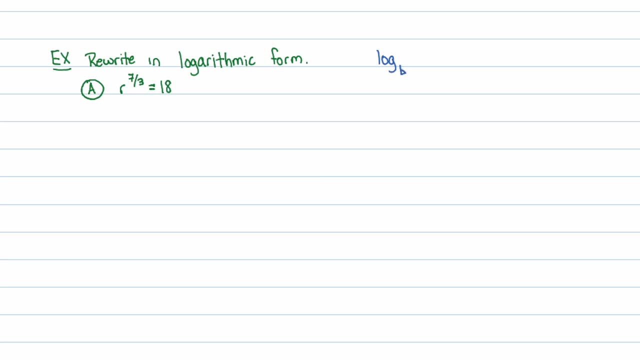 me use blue for that is that log base b of x is equal to y really does imply- and I did a double implication because it goes both ways- that b is equal to y. So I'm going to write b to the y power is equal to x And that's using the circular argument b to 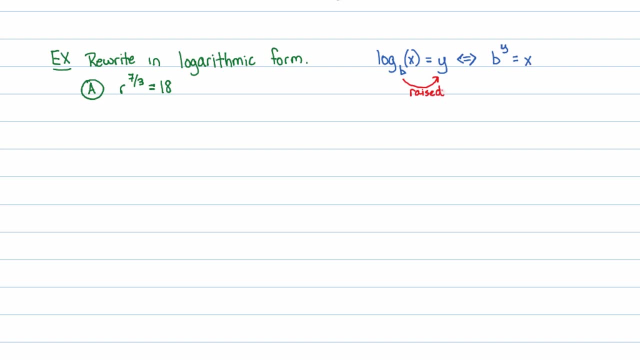 the y power. so I'll write: raise two and is equal to x. So let's transform this into a logarithmic equation. Let's see, that means I'm given this form right here and I just match up the letters on here with the letters on the log. 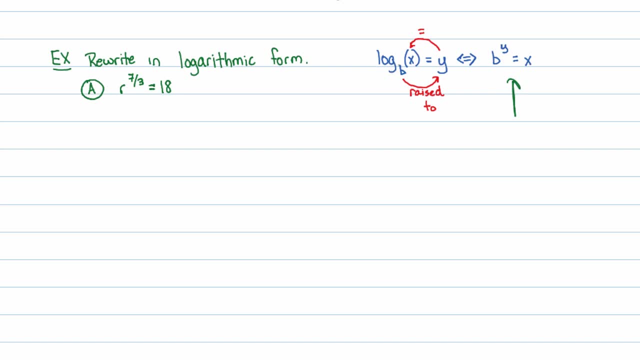 The base of the exponent is also the base of the log. That's probably the best thing to remember. So the base of the exponent is going to be the base of the log. The base of the exponent here is just r, So the base of the log should be r as well. Go ahead and. 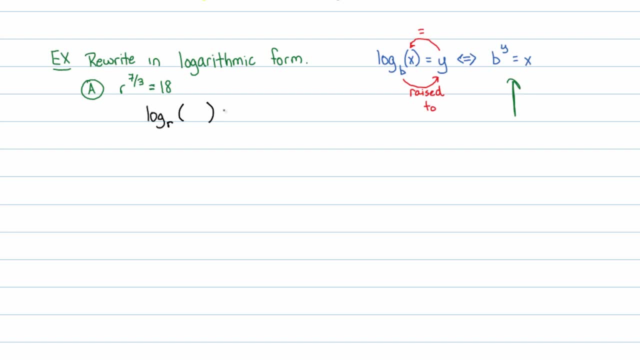 write that in And then I have of something equals something. Then I think about the circular argument. R raised to goes here. So whatever I'm raising r to should go on this side And let's see what am I raising r to. I'm raising r to seven thirds, So r raised to seven thirds and again using the 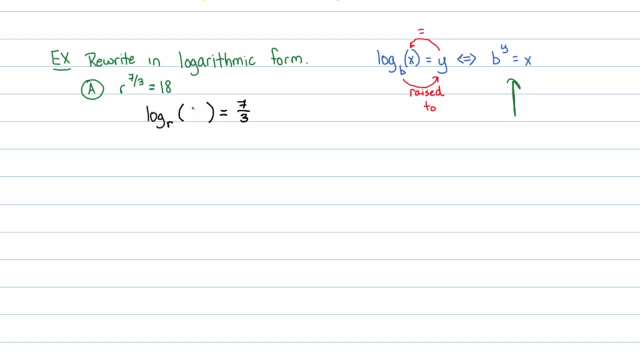 circular argument should equal the inside of the parentheses. Look at the try to do the circular argument here. r raised to the seven thirds is equal to 18.. Is that what that says? Yes, it is. R of this is log base. r of 18 is equal to seven thirds. Now, because this is so new. 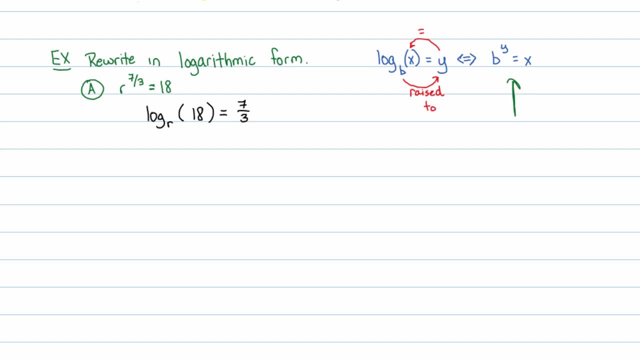 I need to warn you, All you're doing- you're not solving for r here. All you're doing is rewriting this into a different form. The reason why is because you have to get to know this form first. You have to really get pretty good working knowledge of logarithmic form. 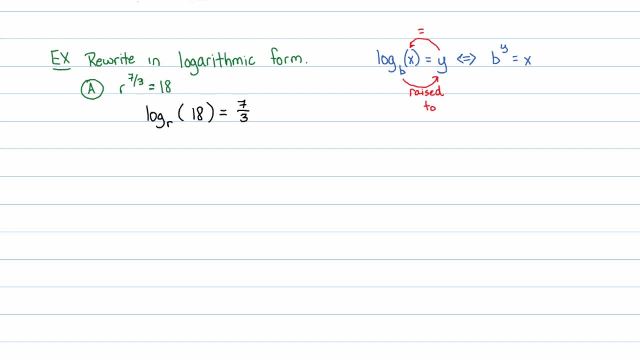 and how to transfer between logarithmic form and exponential form. So that's what we're just playing with here. We're not trying to solve for r or anything like that. Let's do another example, sample b. So we have y to the four, x power is equal to three. 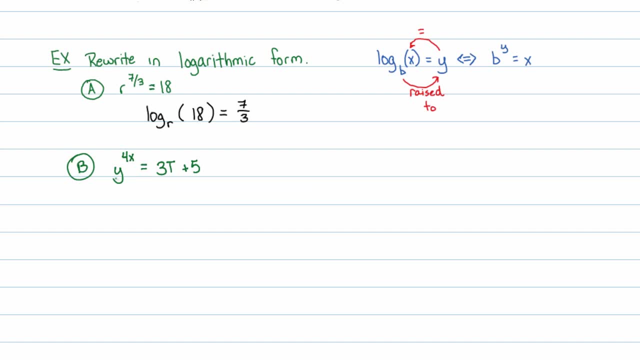 t plus five. It's okay to have a bunch of variables in these problems. All I want to do is rewrite this in logarithmic form. Well, the base of the exponent is y, so that will be the base of my logarithm. I'll write log: base y of something equals something In thinking about. 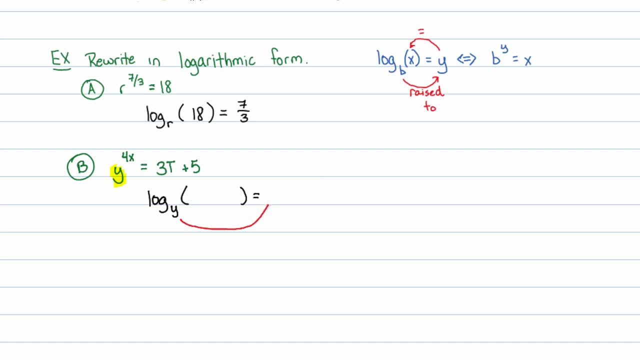 the circular argument. as always, I'll say: y raised to that power. right, there should equal the inside. Well, what was y raised to The 4x? So I'm going to put 4x over here, y raised to the 4x. And then again the last arrow, the over arrow, says what it's equal. 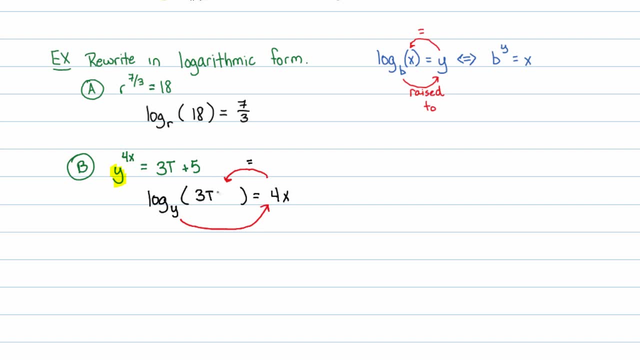 to. It's supposed to be equal to 3t plus 5.. And here we have a great logarithmic equation here: Log base y of 3t plus 5 is equal to 4x. Technically that's saying the same exact. 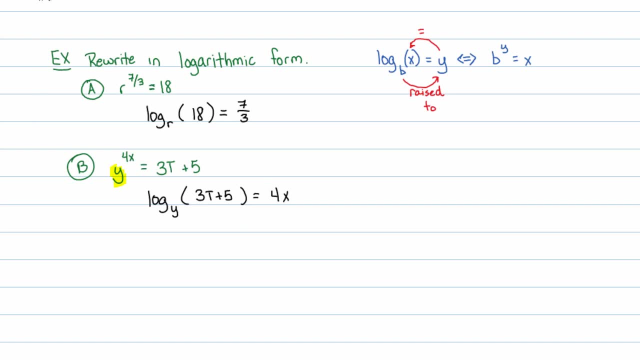 thing as y to the 4x. Y to the 4x is equal to 3t plus 5.. Just one is written in logarithmic form and one is in exponential form. Now I really started this off on the harder way of doing things. 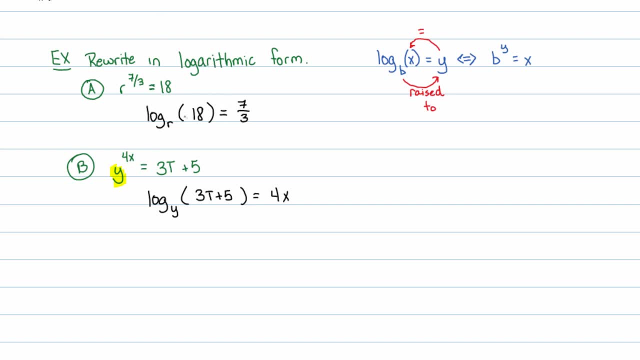 because honestly, I think transforming from logarithmic form back to exponential form is very easy. You'll see why. Suppose I give you log base b of 9 is equal to negative 2. And I say: please rewrite this in exponential form. That means I'm just going to say b raised. 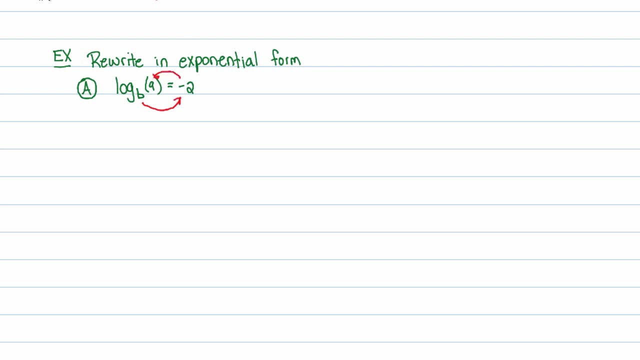 to the negative 2, power should be equal to 9.. So I'll just write out what I just said: b raised to the negative 2, power should equal 9.. Now remember, they didn't ask me to solve, They just asked me to rewrite this in exponential form. So I'm done. Don't go any further, You. 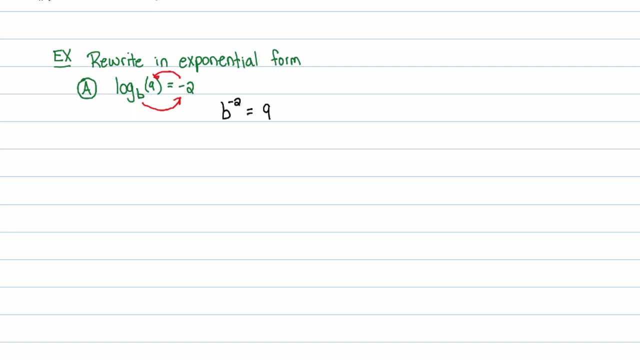 could solve for b, but I don't want to. Let's just pretend that this is where we're parking it. For example, part b, log base 4 of 36 is equal to 2q minus 1.. Again, all we're doing is: 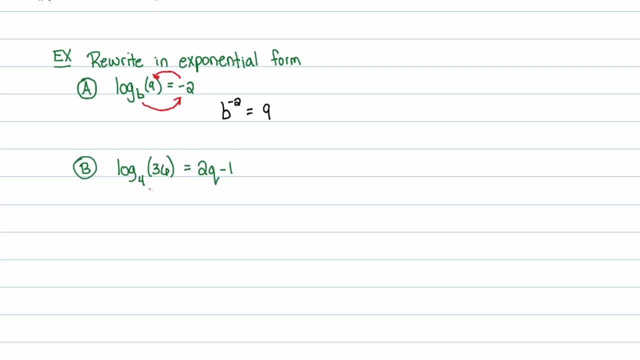 rewriting this in exponential form, And I just use my circular argument: 4 raised to this junk is equal to 36.. So I'll use a little caret sign, meaning raise there. So let's go ahead and write that down: b raised to the 2q minus 1 should be equal to 36.. And that's all they want me to do is just. 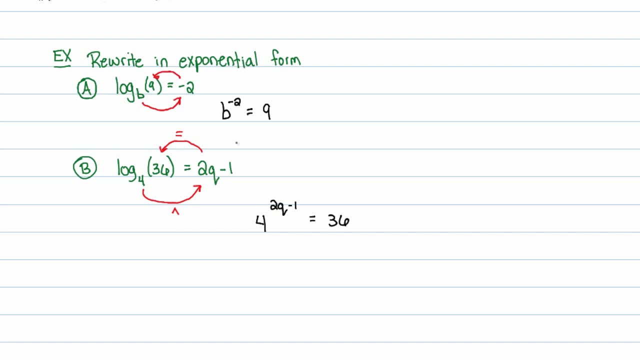 to stop there. That is written in exponential form. No need to try to solve That one would be a wonderfulness to solve, but don't do it Now. I thought I would continue in this video to evaluate logarithms, but I think this is.